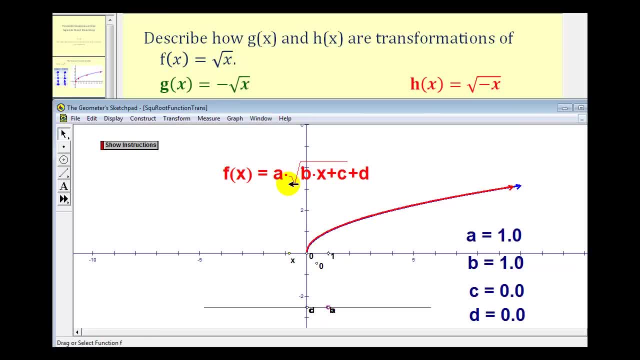 To analyze g of x. here we'll change a to negative 1.. So the basic square root function will be blue and the transform function will be in red. Notice, as we change a to negative 1, the red function is now a reflection across the x-axis. 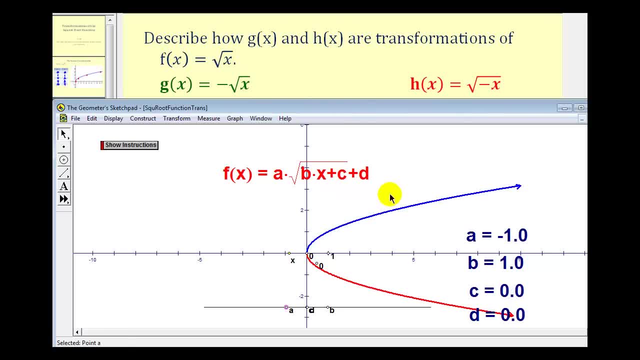 So the function g of x equals negative square root. x changes the sign of the y coordinates of the parent function to negative, producing a reflection across the x-axis. Now to see how h of x equals square root, negative x transforms the parent function, we'll change b to negative 1.. 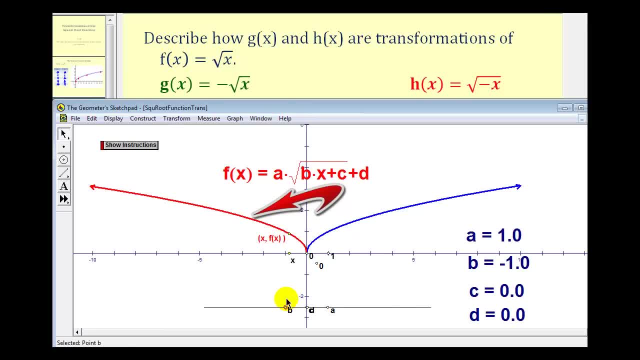 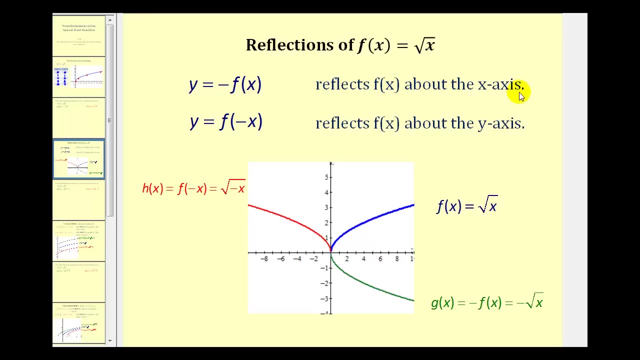 Notice, when b is equal to negative 1, we now have a reflection across the y-axis. This negative in front of the x here changes the sign of all of the x coordinates of the parent function, producing a reflection across the y-axis. So to summarize this: if y equals negative f of x, we have a reflection about the x-axis. 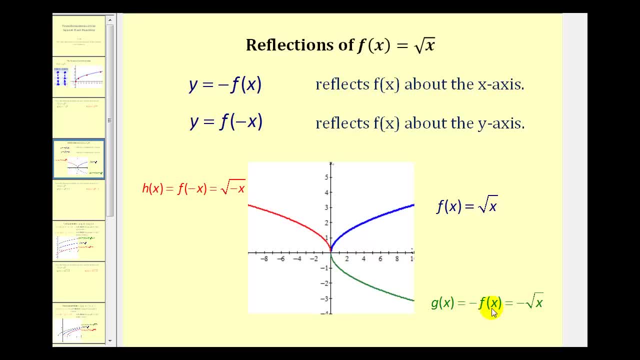 which we have here in green, where g of x equals negative f of x, which is equal to negative square root x, And if y is equal to f of negative x, this reflects the function across the y-axis which we have here in red. h of x equals f of negative x. 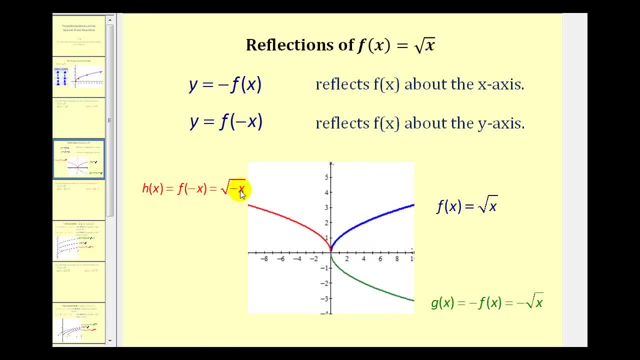 which is equal to the square root of negative x. So here the effect is changing the sign of the x coordinates of the parent function, and here the effect is changing the sign of the y coordinates of the parent function. Now let's consider: g of x equals the square root of x plus 2,. 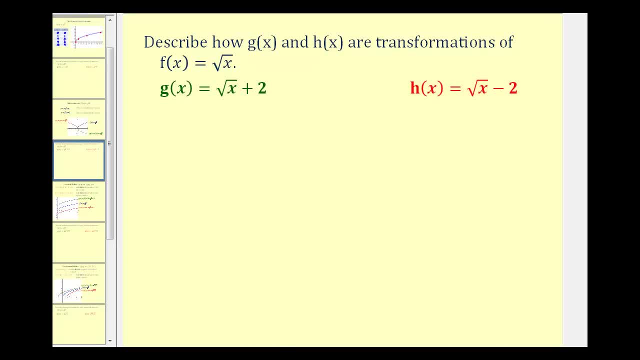 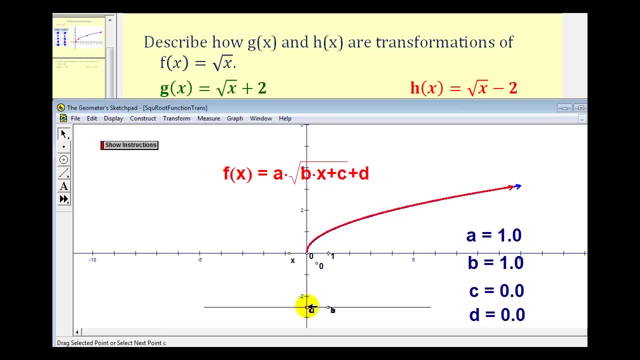 and h of x equals the square root of x minus 2.. Notice, in this case we'll be changing the value of d to plus 2 and minus 2.. Notice, as we change d to positive 2, the function is shifted up two units. 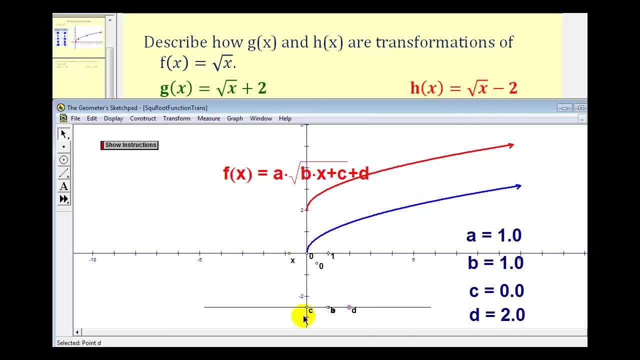 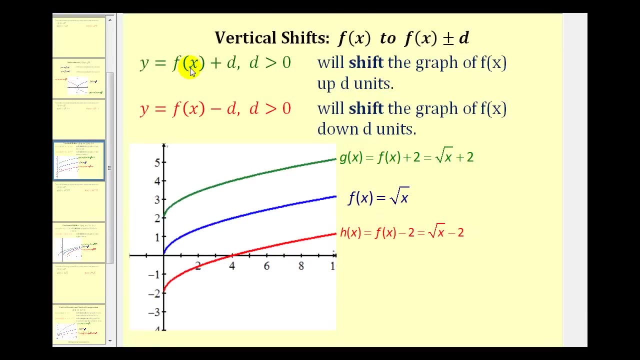 And for h of x equals the square root of x minus 2, we'll change d to negative 2.. Notice, when d is equal to negative 2, the function is shifted down two units. So to summarize this, if we have y equals f of x plus d, 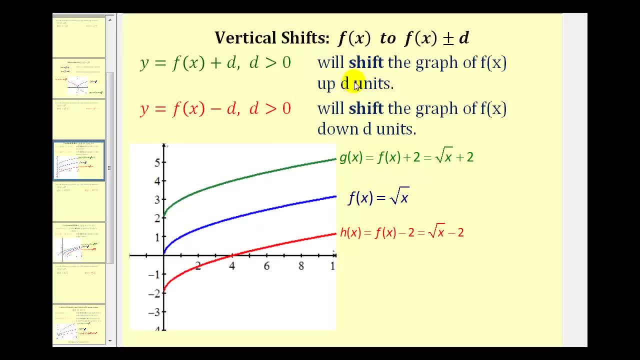 where d is positive, the parent function will be shifted up. d units, as we see here in green: g of x equals f, of x plus two would be equal to the square root of x plus two. And then, if we have y equals f of x minus d. 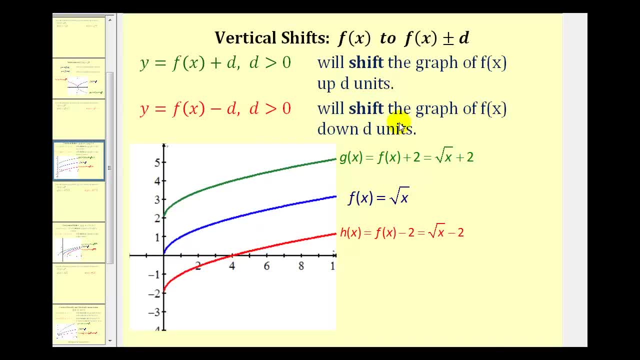 again, where d is positive, we would have a shift of the function down d units, which in our case is: h of x equals the square root of x minus two, which is equal to the square root of x minus two. Next we'll consider g of x equals the square root. 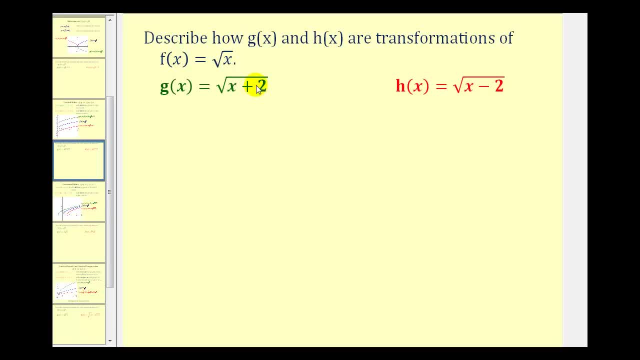 of the quantity x plus two. Notice how the plus two is underneath the square root now. and h of x equals the square root of the quantity x minus two. Again, the minus two is underneath the square root. So to see how this affects the parent function. 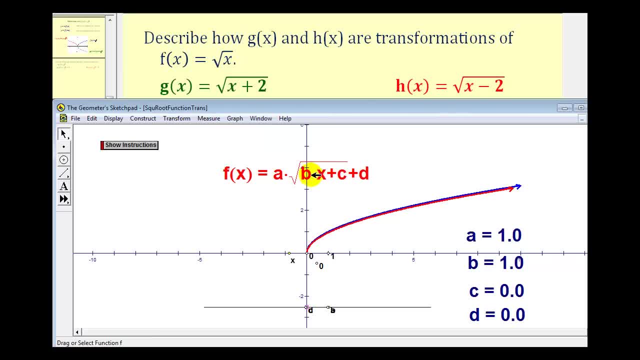 notice how now we'll be changing the value of c, while b is equal to one. So as we change c to positive two, notice how now the function is shifted left. so when c is equal to positive two, we have a horizontal shift left two units. 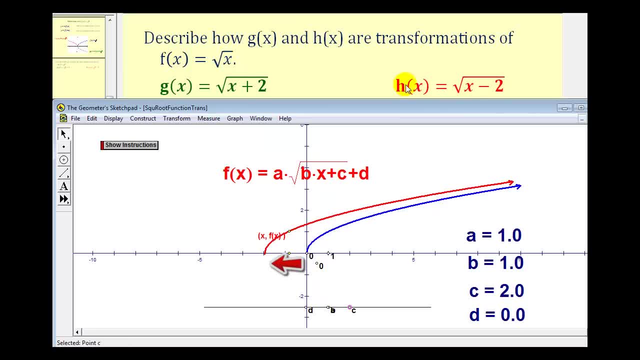 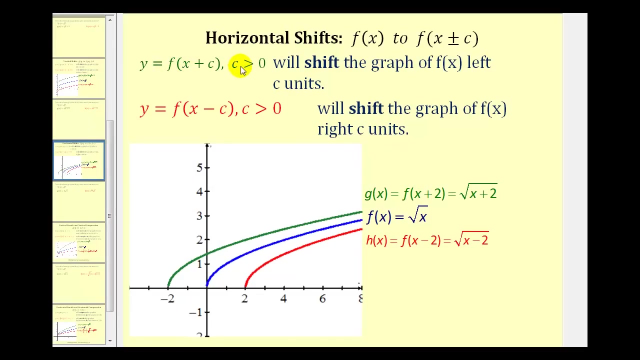 And for h of x, we'll change c to negative two. Notice how now the parent function has been shifted to the right. So again, let's go ahead and summarize this transformation. When y is equal to f of the quantity x plus c, 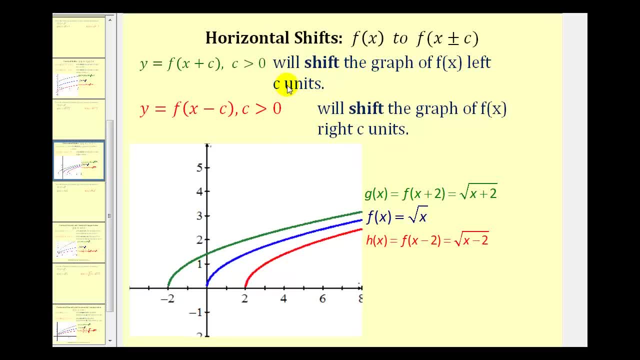 and c is positive, this will shift the parent function left c units which we had here in green. g of x equals f of the quantity x plus two, which is equal to the square root of the quantity x plus two, And if y equals f of the quantity x minus two, 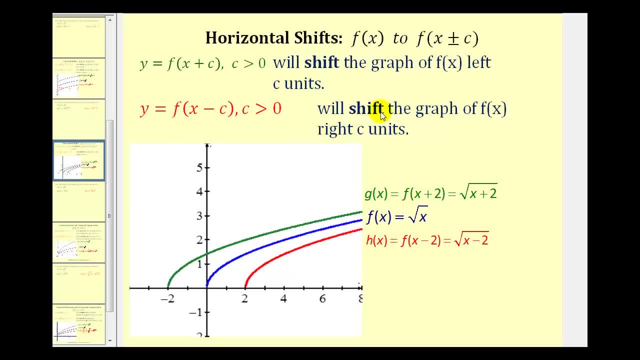 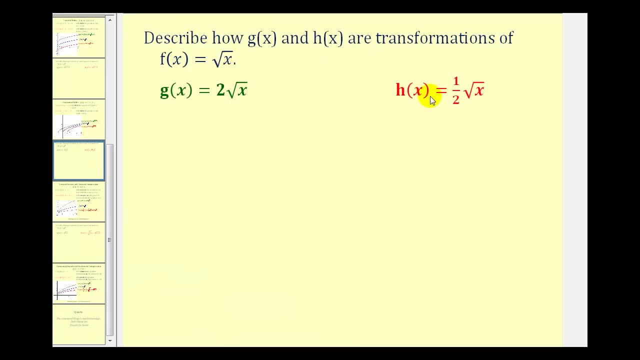 minus c. again where c is positive. this will shift the graph right to c units, where we had: h of x equals f of the quantity x minus two, equal to the square root of the quantity x minus two. Now let's consider: g of x equals two times the square root. 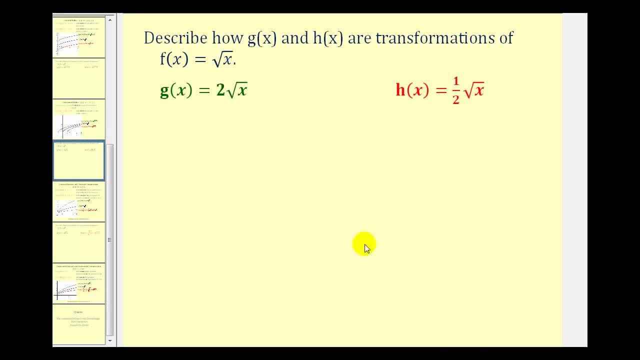 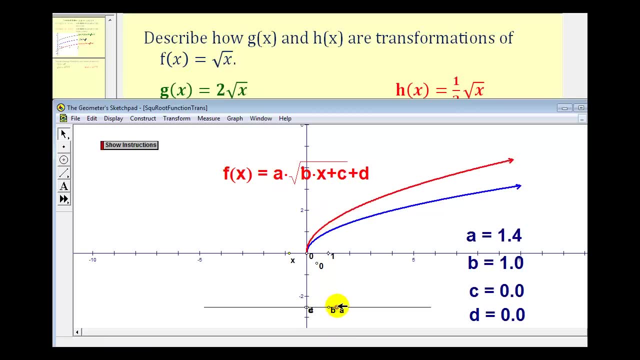 of x and h of x equals one half times the square root of x. So, going back to our animation, we'll now change a to positive two. Notice how, when a is positive two, the graph is stretched vertically because now every y coordinate of the parent function. 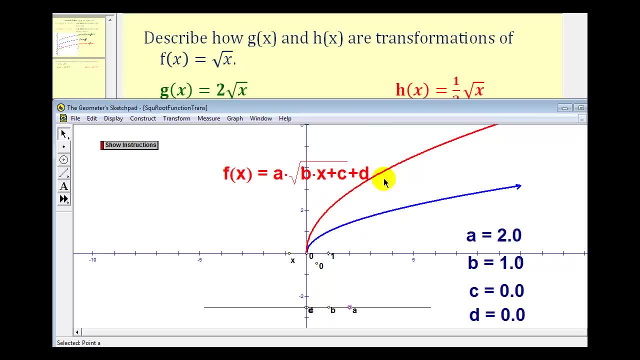 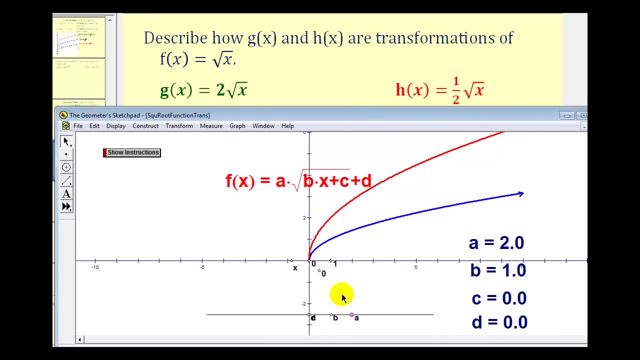 is being multiplied by two. So we call this a vertical stretch. And now for h of x equals one half times the square root of x. we'll change a to one half, Or 0.5.. We'll call it a vertical compression. 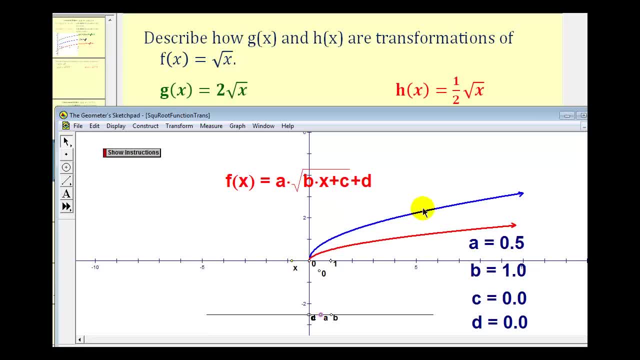 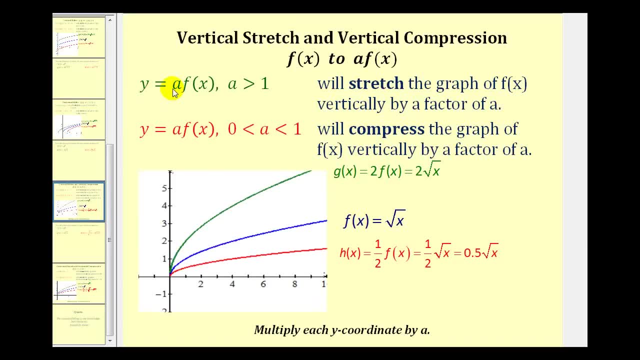 Notice: in this case, every y coordinate of the parent function will be multiplied by one half, which is called a vertical compression. So again to summarize, if we have y equals a times f of x. where a is greater than one, this will stretch the graph. 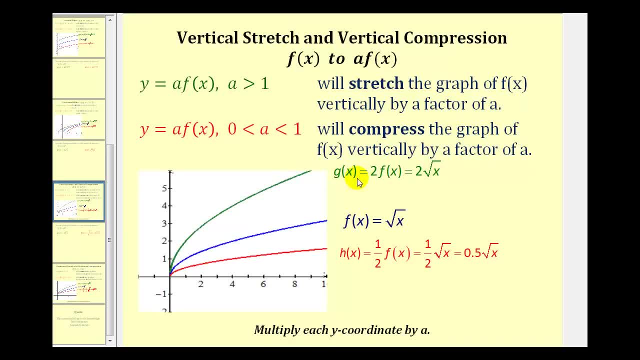 of the function vertically by a factor of a, which we have here in green, And if we have y equals a times f of x, where a is between zero and one, we call this a vertical compression by a factor of a, which is called a vertical compression. 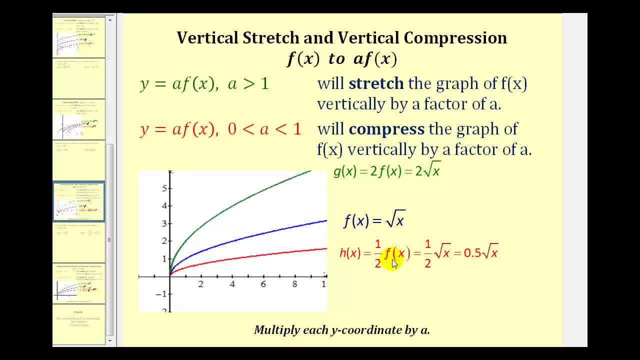 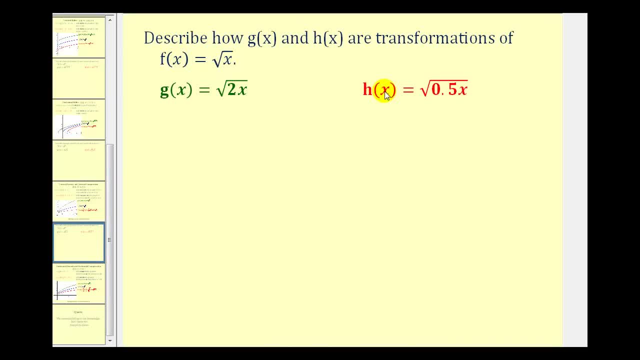 Which we have here for h of x. Now we have one more transformation to consider. Now we want to consider: g of x equals the square root of two x, and h of x equals the square root of one half x or 0.5 x. 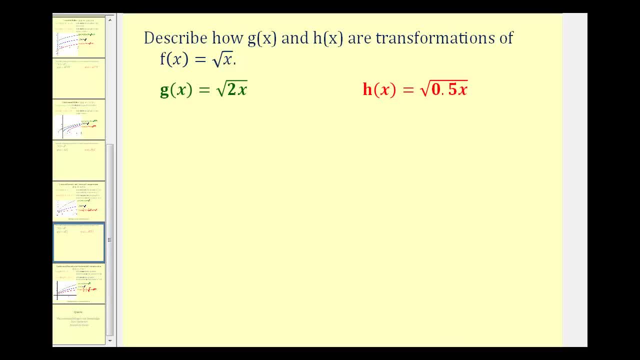 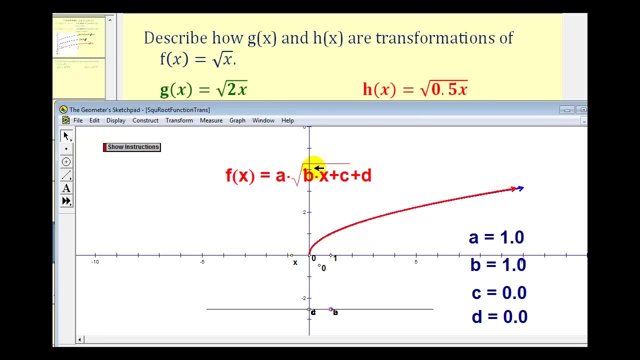 Notice how now the constants are underneath the square root. So, going back to our animation, we want to change the value of b to positive, two for g of x and 0.5 for h of x. So as we change b to two, 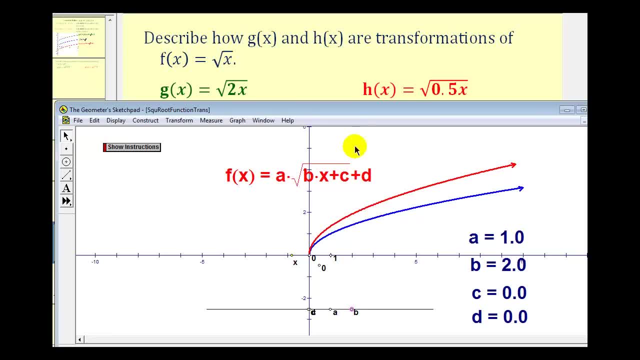 this may appear to be a vertical stretch, but it's actually a horizontal compression. Notice how, if we look at the function x values- that would be half of the parent function- would produce the same outputs as the parent function. Therefore, we call this a horizontal compression. 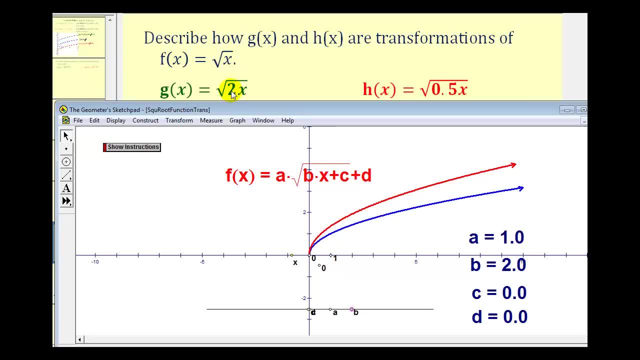 and it's by a factor of one half, the reciprocal of b. Now let's see what happens when we change b to one half Again. this may appear to be a vertical compression, but notice how, now, looking at our function, it would take x values that are twice the x values.